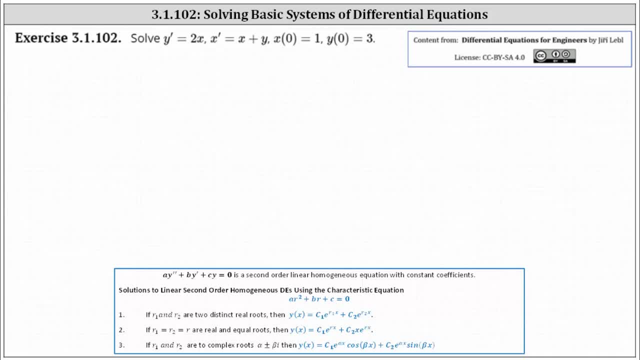 We're asked to solve the system of differential equations: y prime equals two, x and x prime equals x plus y. with initial conditions, x of zero equals one and y of zero equals three. Both x and y are functions of t. Beginning with the first equation, y prime equals two x. 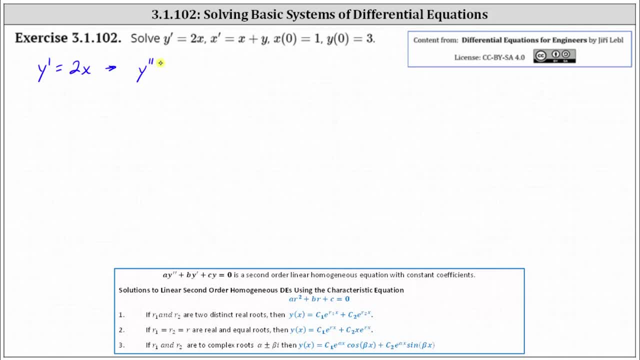 If we differentiate both sides with respect to t, we have: y double prime equals two x prime. And now, using the second equation, we know x prime is equal to x plus y, which gives us y double prime is equal to two times the quantity x plus y. 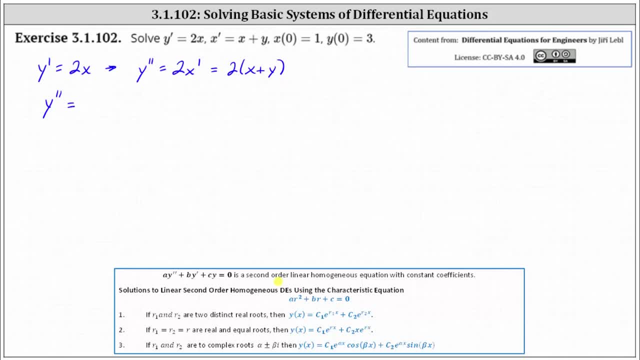 Distributing we have: y double prime is equal to two x plus two y. And now going back to our first equation, we know y prime is equal to two x and therefore we can write the differential equation as: y double prime equals y prime plus two y. 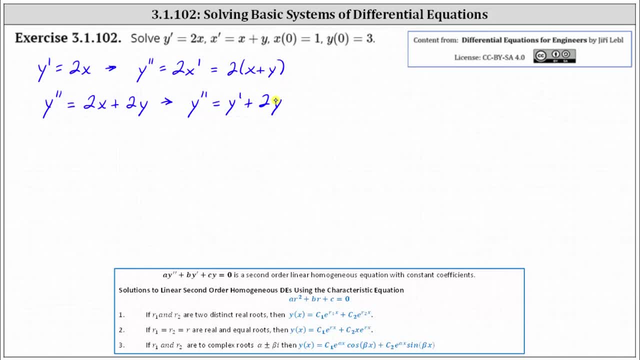 We should recognize this as a second-order linear, homogeneous differential equation with constant coefficients And therefore we can solve this using a characteristic equation. but we first need to set the right side of the equation equal to zero by subtracting y prime and subtracting two y on both sides. 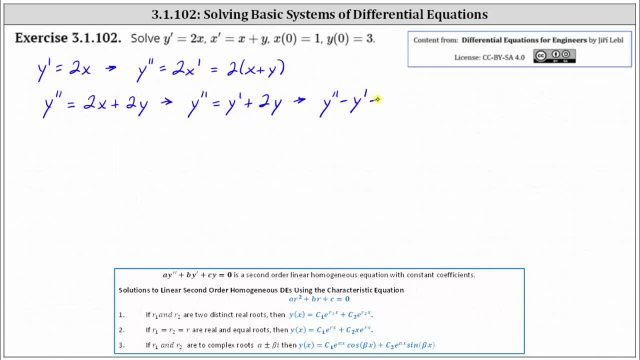 This gives us y double prime minus y prime minus two. y equals zero, And the corresponding characteristic equation is r squared minus r minus two equals zero, which we can solve by factoring the factors of y prime. So we have r squared or r and r. 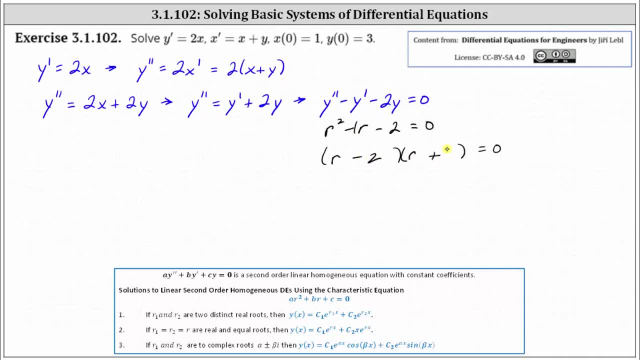 The factors of negative two that add to negative one are negative two and positive one, giving us roots or solutions of two or negative one. Because we have two distinct real roots, the general solution is in the form of, in our case, y of t. 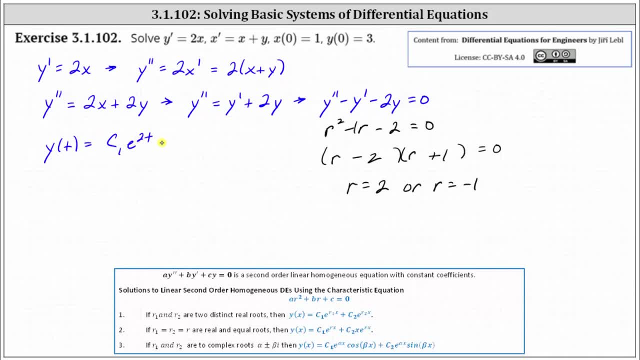 is equal to c, one e to the two t plus c, two e to the negative t. Now let's work on determining x of t. We know from the first equation that y prime is equal to two x Multiplying both sides by one half. 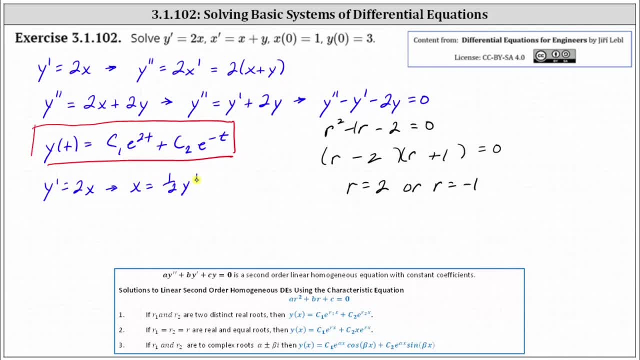 we have, x equals one half times y prime, And since we know y, we simply need to determine y prime, then multiply by one half. So x or x of t is equal to one half times y prime. Y prime is equal to c one, e to the two t times two. 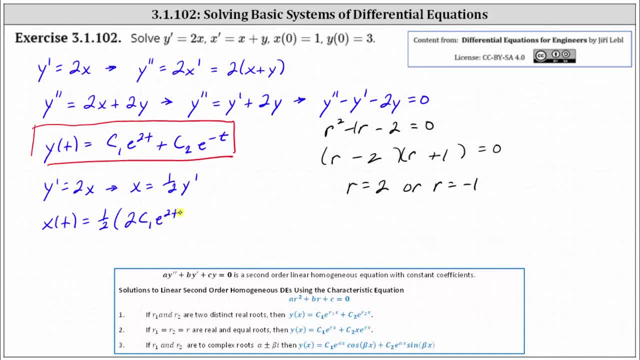 or two c one e to the two t and then plus c two e to the negative t. times negative one or minus c two e to the negative t. Distributing we have x of t equals c one e to the two t. 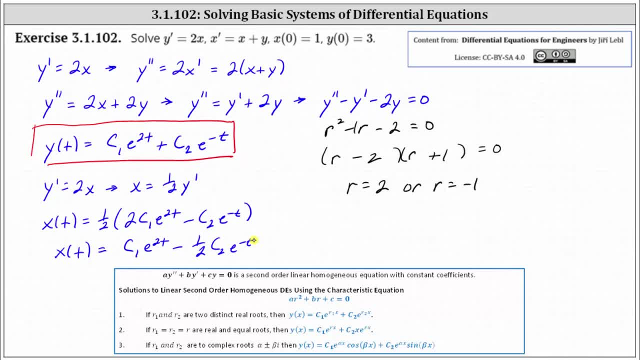 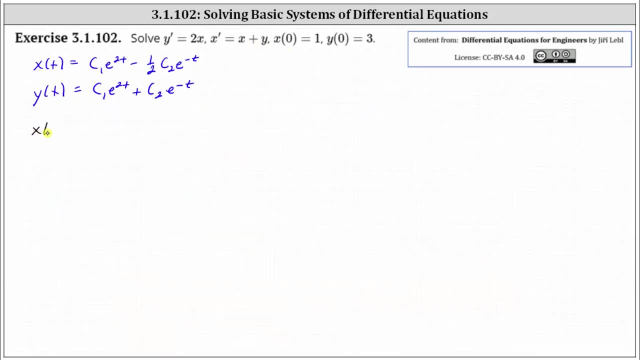 minus one half c two, e to the negative t. Now that we have the general solution to the system of differential equations, we now need to determine c one and c two using the initial conditions. Let's do this on the next slide. Using the initial condition, x of zero equals one. 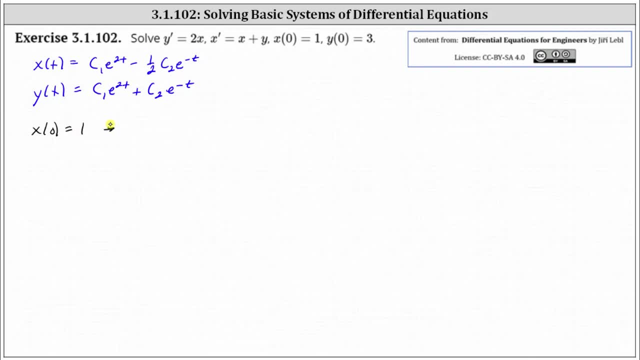 in the equation for x, we substitute zero for t and set the function value equal to positive one. This gives us c one, e to the zero minus one half c two e to the zero equals one. Simplifying, we have c one minus one half c two equals one. 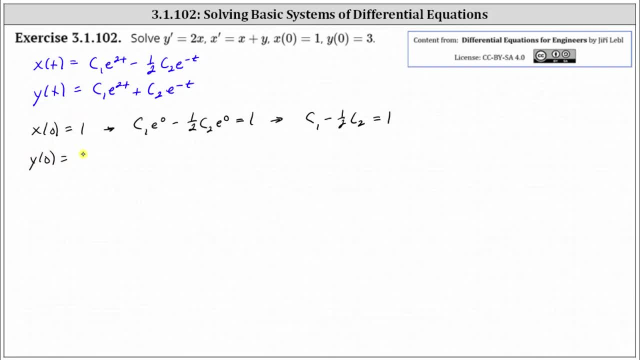 And now using y of zero equals three. in the equation for y we substitute zero for t and set the function value equal to positive three. This gives us c one. e to the zero plus c two. e to the zero equals three. Simplifying, we have c one plus c two equals three. 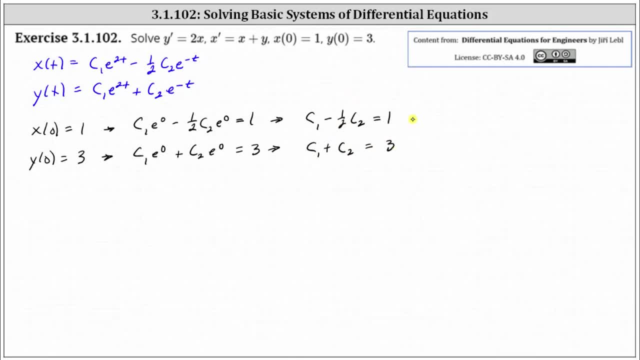 To solve the system. let's go ahead and multiply the first equation by positive two, so the c two terms are opposites. This gives us two c, one minus c. two equals two. Leave the second equation the same. Add in the two equations together. 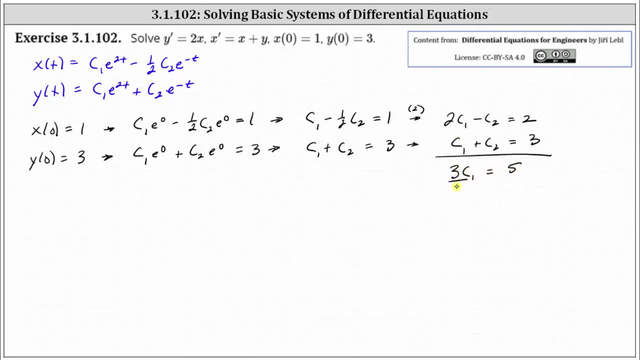 we have three. c one equals five, Dividing both sides by three. we have c one equals 5, 3rds. Well, if c one equals 5 3rds and c one plus c two is equal to three, which is 9 3rds. 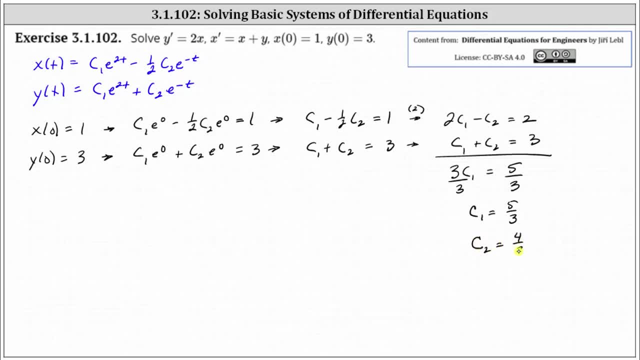 we now know c two is equal to 4 3rds. And now we go back and substitute 5 3rds for c one and 4 3rds for c two. This gives us x of t is equal to 5 3rds, e to the two t. 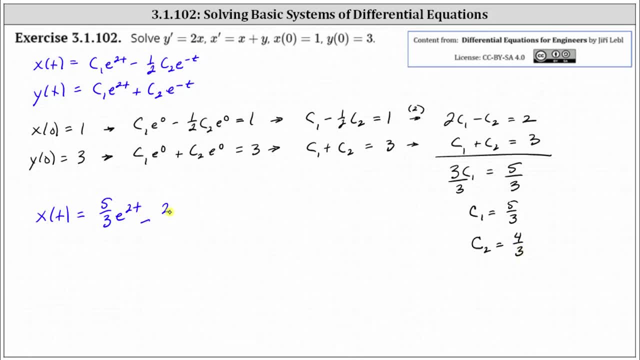 and then minus 1 1⁄2 times 4 3rds is 2 3rds, giving us minus 2 3rds e to the negative t, And for y of t we have: y of t equals 5 3rds e to the two t.